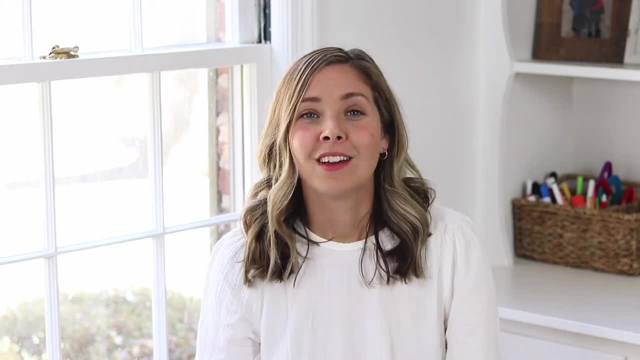 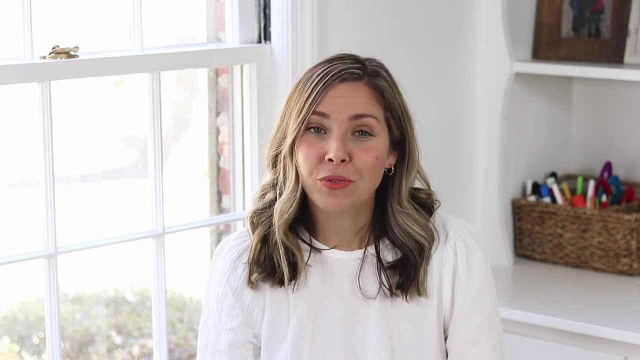 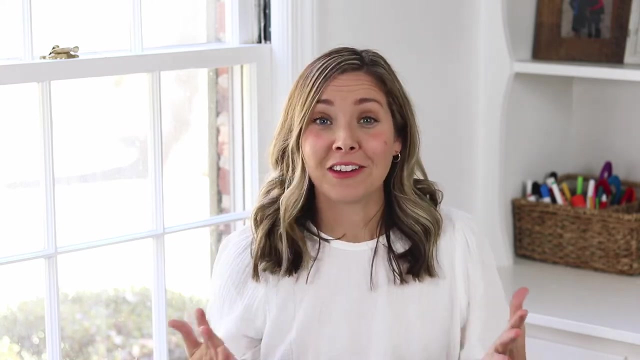 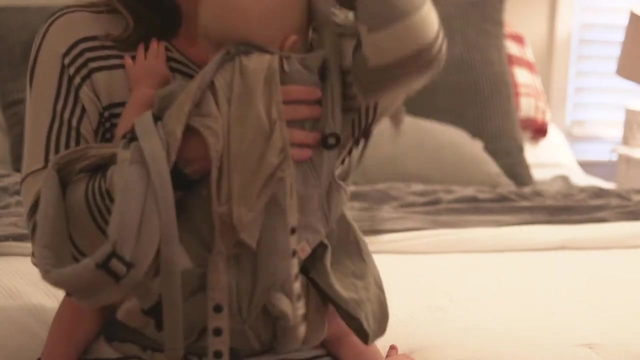 I'm going to show you how to get things done with a baby. So welcome to this channel. My name is Lena and this is Girl Teach Me. I also run GirlTeachMecom, which is a blog for new moms with real food recipes and lots of strategies to create a peaceful home for the people that you love, And if any of that resonates with you, I hope you'll hit subscribe. Okay, so the first strategy I have for getting something done is baby wearing. I am obsessed with baby wearing. I love it and I know it can hurt your back. at first. I think there's a better way to do it if it is hurting your back, But sometimes 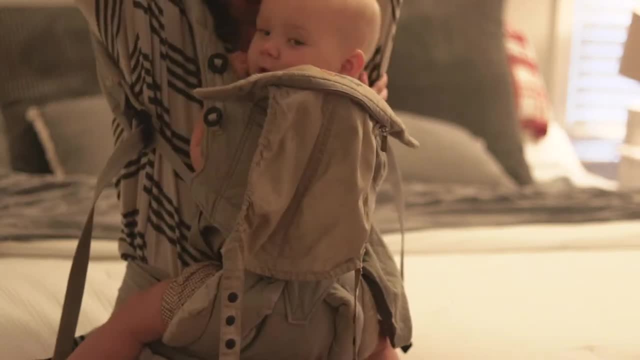 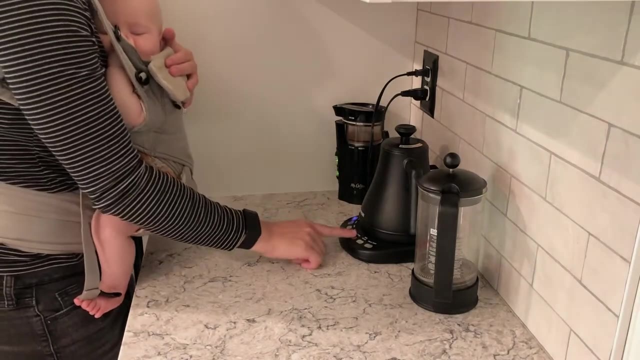 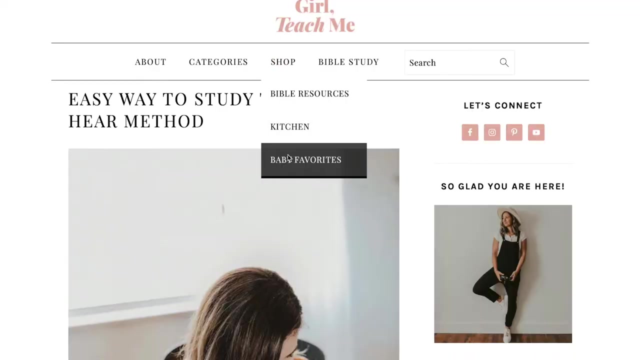 your back just has to get a little bit strengthened up to baby wearing. So maybe it's just in 10 minute, 15 minute spurts. I think the Ergo is my absolute favorite. I actually have a list of my baby favorites over on Girl Teach Me, just to help you if you're a new mom and you just are like 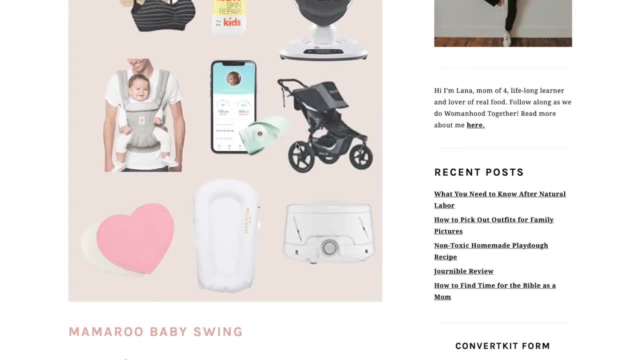 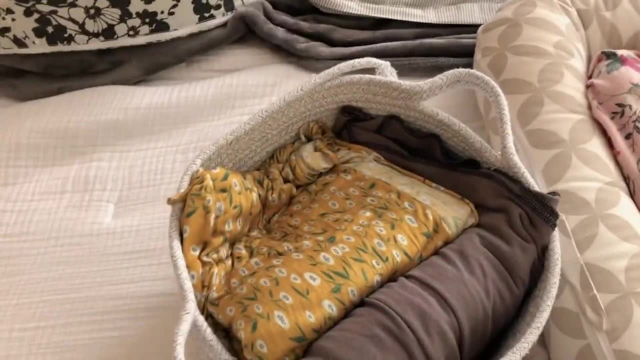 I don't know what I should have had on my registry but don't. I don't know what baby wrap to get. I like the Moby when they're super little. I like the Ergo for getting stuff done, And the other ones are pretty and nice to wear to church. 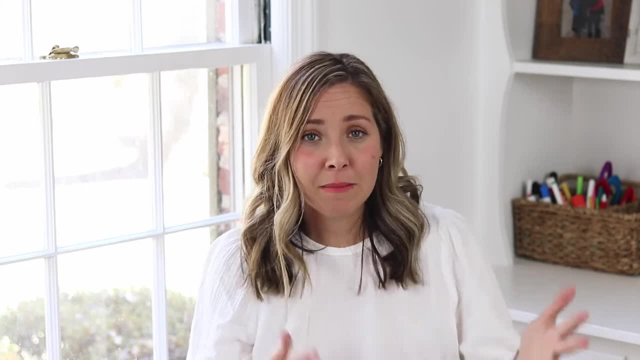 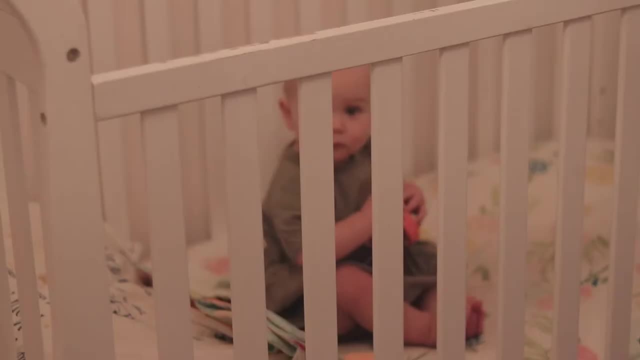 The second thing I would say is just some alone time, Like let the baby be alone, Let the toddler be alone. Everybody needs a little bit of alone time. So that might look like them literally being in their crib awake for 10 minutes. You're not breaking your connection. You're not breaking. 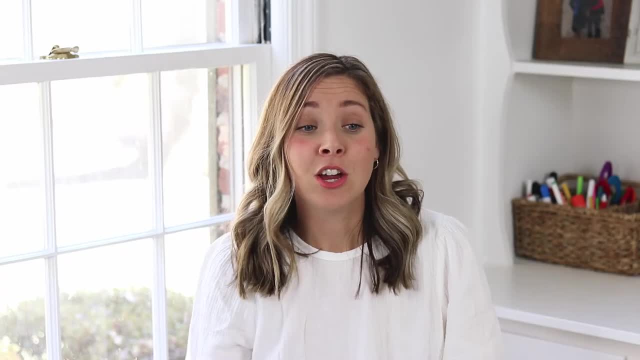 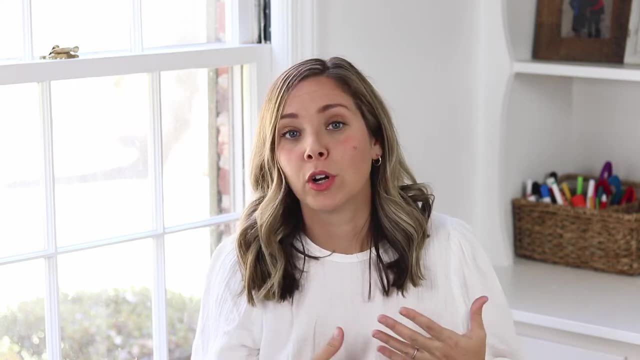 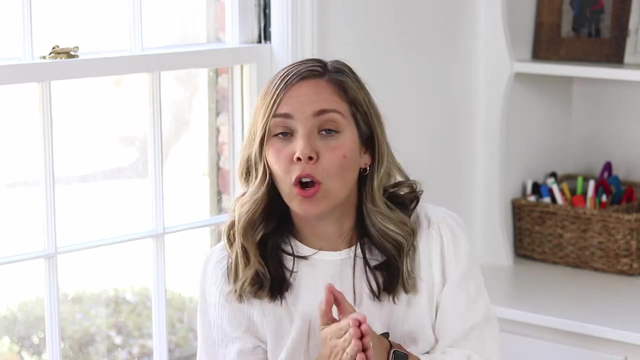 your bond, You're getting a moment to yourself, You're getting some sanity. So maybe that looks like you set a 10 minute timer. You give the child an age appropriate toy or no blankets or no toys, and they just are sitting there and just being quiet for 10 minutes. In 10 minutes you go and 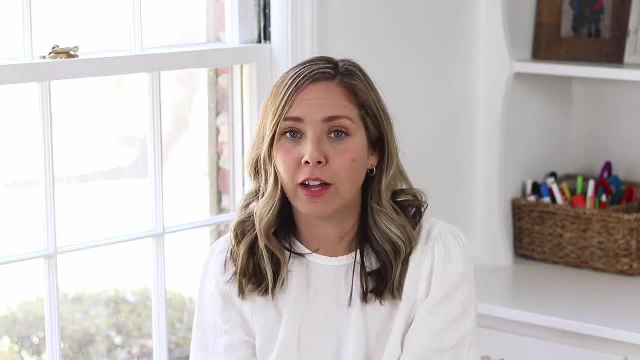 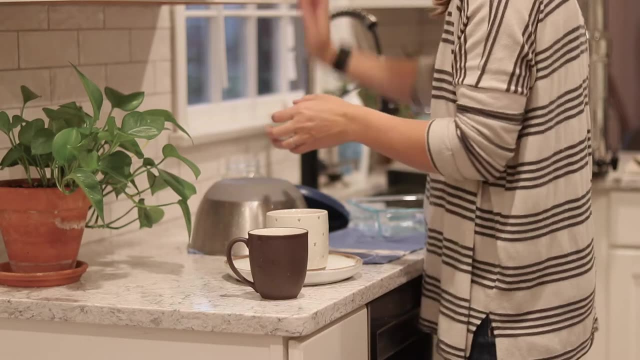 you go get your shower, Or 10 minutes you go and you blow dry your hair, Or 10 minutes you go and you do those dishes. I am all about my third point: timers. Timers are an absolute lifesaver. as a mom, I live and die by my timer. I love my. 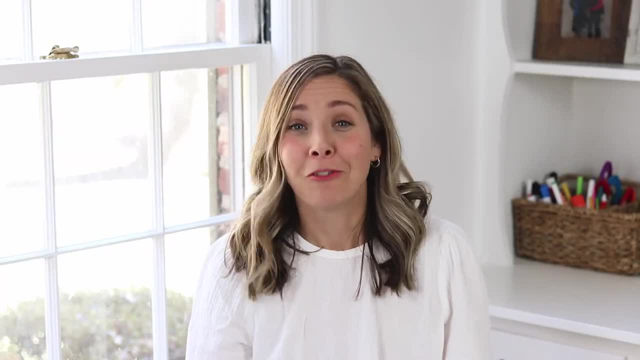 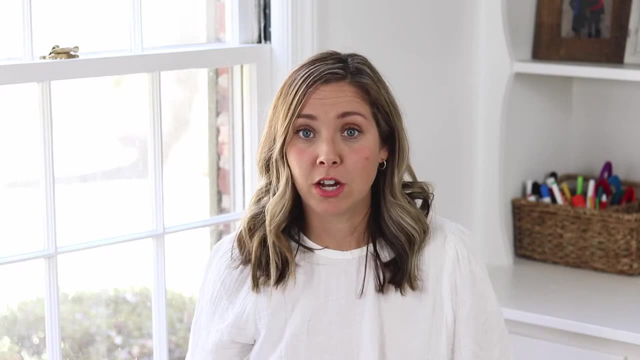 Apple Watch for a timer. I love my oven for a timer. I'm setting a timer all the time. It's my number one productivity tip. So I feel like when we have a start and when we have a stop, we work a little bit more efficiently. And it's kind of like you think if you had more time, you'd be more. 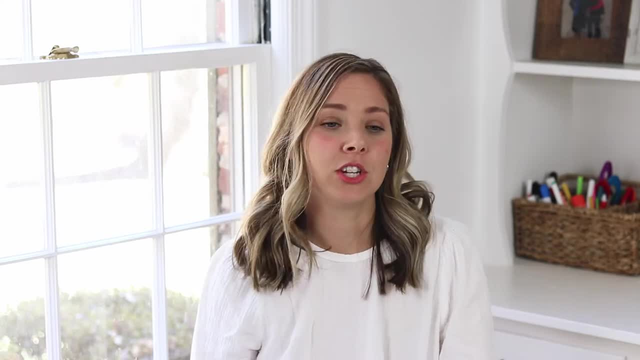 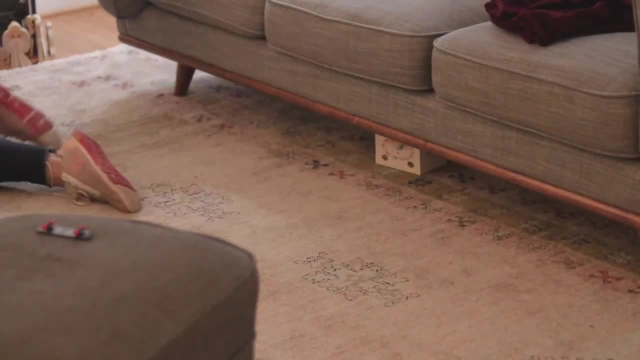 efficient. but it's not true: If you have less time you will be more efficient. So if you really need to get something done, I say: set a timer. Be realistic about the fact that if you used to dawdle when it came to cleaning before you had time to do it, you're not going to be able to. 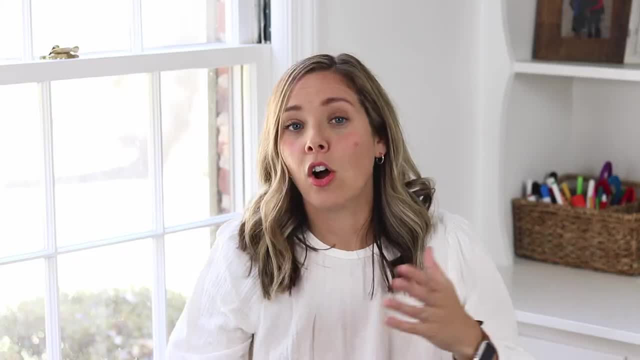 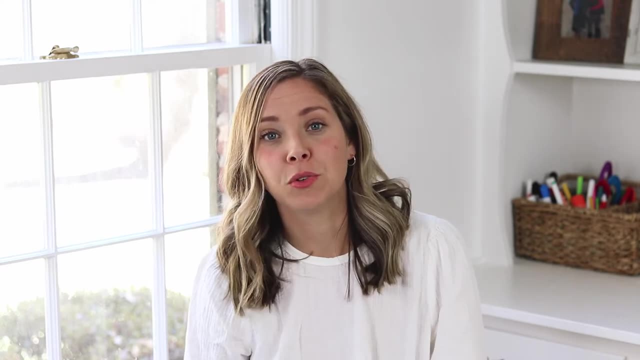 do that anymore. If you used to dawdle and get all of the accoutrements right before you got into the word, you can't do that anymore And I actually. it might be a gift to you. You might find that. 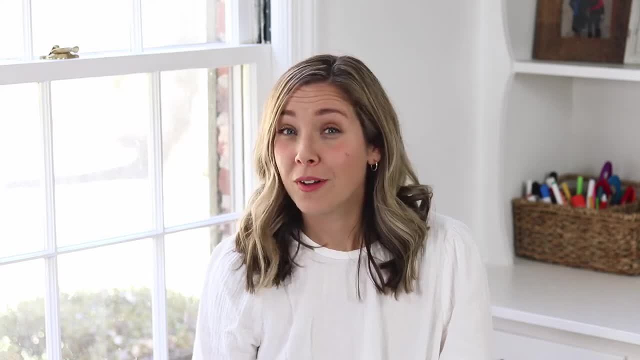 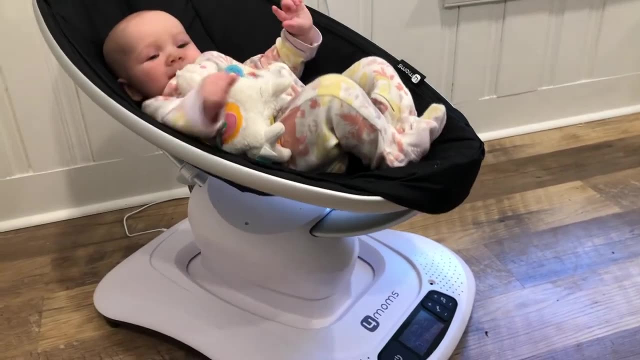 you're far more efficient. So set a timer. It's my favorite. The fourth thing I would say is the baby swing. If they are young enough to be put in a baby swing, they absolutely love it. If they're a little bit older, maybe it's their high chair with some food to play with. Yes, you might have. 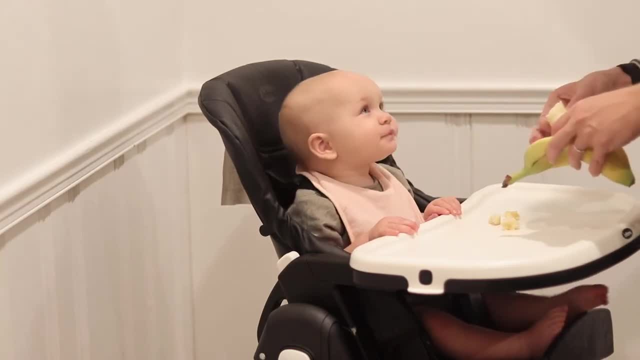 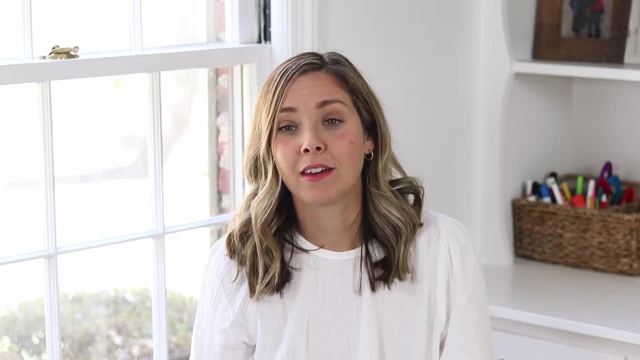 to wait for them, and it's a mama break from you having to hold them all the time. What I want you to understand is: you're not a bad mom if you set your kid down. You're not a bad mom if you take a break. Yeah, you might be a bad mom if you leave your kid unattended for eight hours. I'm not saying 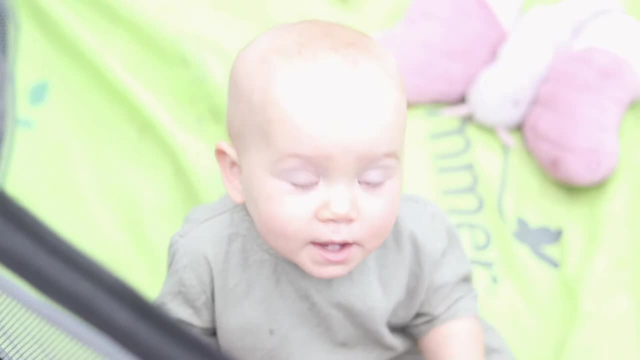 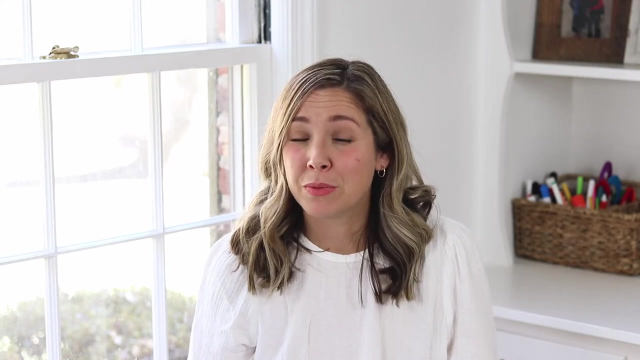 that What I'm saying is just for a moment in time. if they're in a safe place and you know they're okay, take a moment to yourself. The next thing I would say is maybe a mom swap. I am literally doing a mom swap so I can do this video. If you have kids that are having fun in the kitchen, you could go. 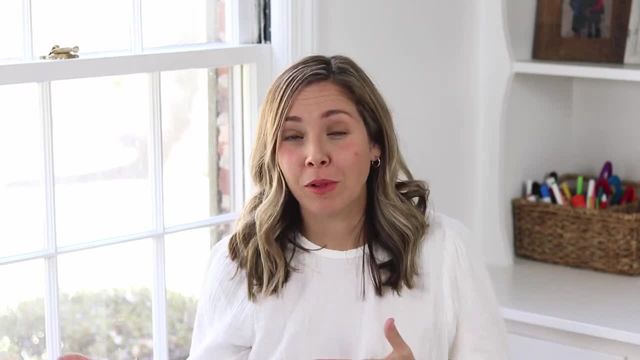 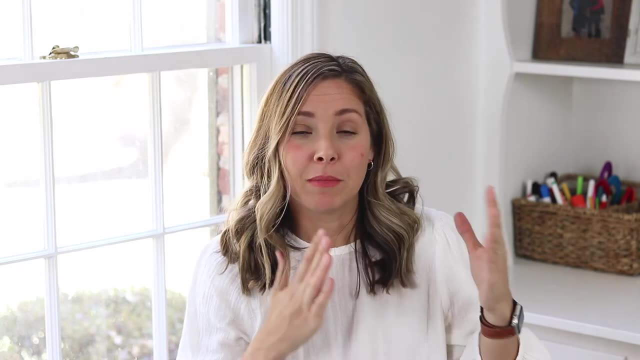 video right now. Um, I keep my friend's kids for a couple hours one time a week. She keeps my kids for a couple of hours one time a week. They get some kid time. I get a break, My friend gets a. 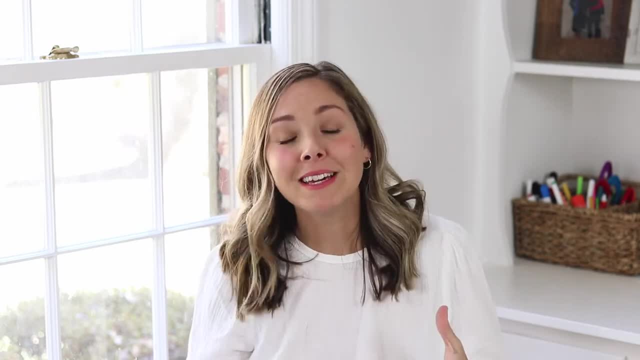 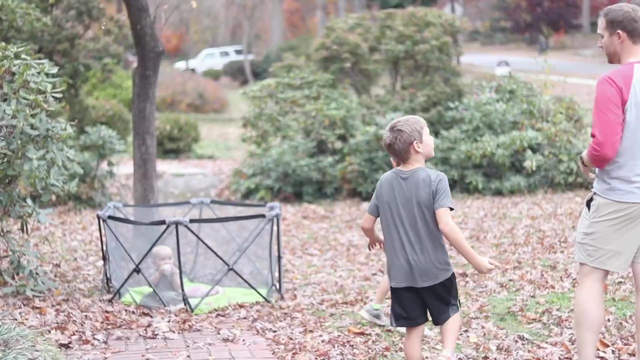 break. She does whatever she wants. I do whatever I want. So maybe consider a mom swap. Maybe consider, um, just letting dad watch the baby for a second. Like I know, some moms don't want to let anybody else bond with their baby, Anybody else hold their baby. But I really think babies are. 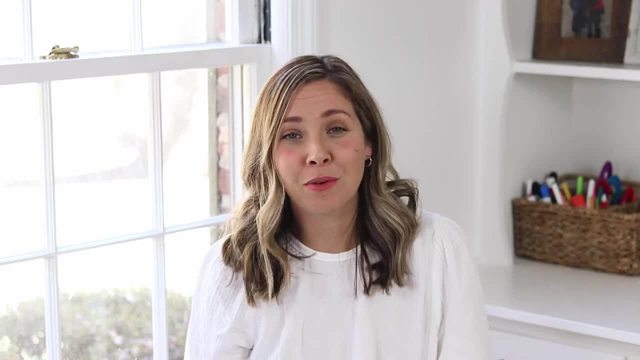 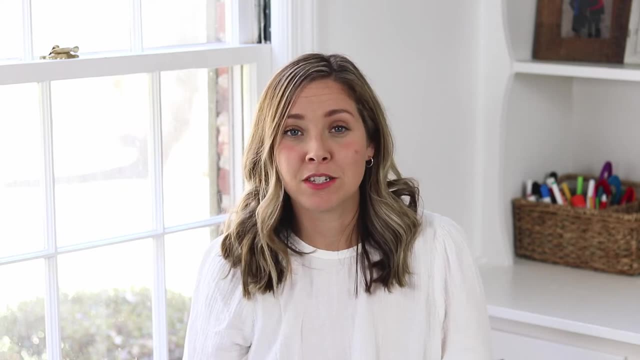 meant to be shared. They're so precious and so wonderful. Daddy needs to bond with baby too. So you know, maybe it's just letting somebody else help you and getting a moment to bust a move. I'm telling you what, if you used to work out? find a way to work out, Even if it's just gently. 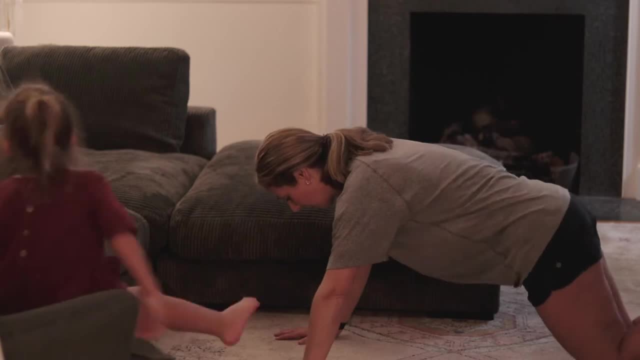 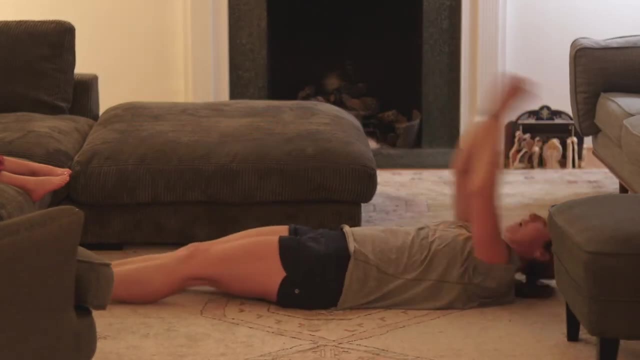 moving. it's going to help you feel more like yourself. If it was going to a coffee shop to get into the word, do it. It's going to make you feel more like yourself. So just find a way to get back to some of the things you loved that. 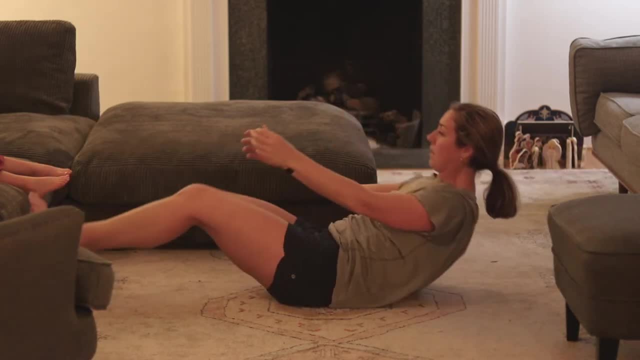 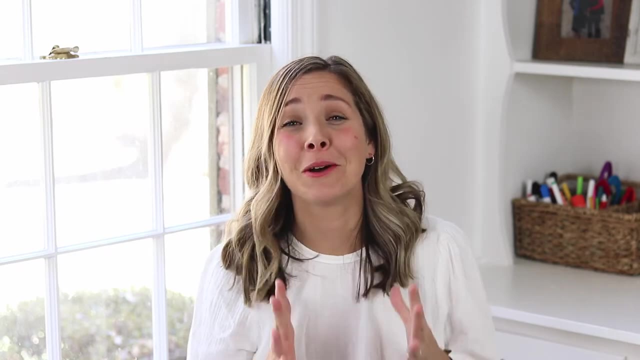 made you feel more like yourself? Maybe not, are not even productive. just to make you feel more like yourself, It's going to help your new mom overwhelm your new mom, depression and anxiety. It's just going to help so much to get back to some of the things you love. And if you love being productive, set those timers and 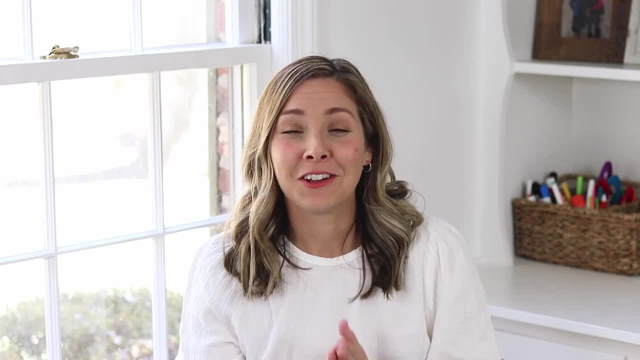 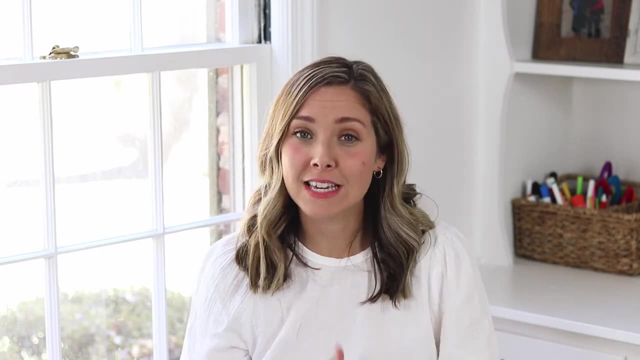 get back to it. A word on feeling like a failure. You are just not going to be able to do all the things you used to do And I'm sorry I know that's so hard to hear, but it's a season, It's. 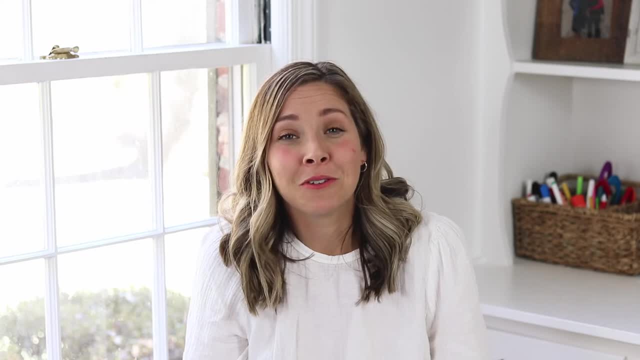 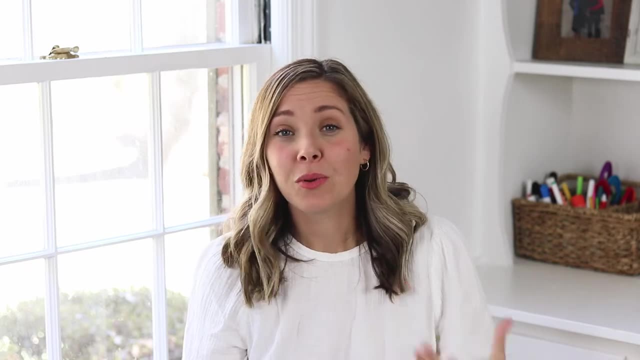 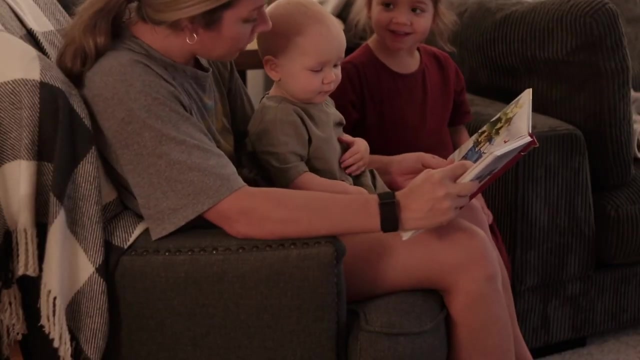 going to be hard, But you can do more, And so you need to be aware of everything that you've done, that really, what you're, what you are allowed and supposed to be doing right now, is staring at your baby, enjoying your baby baby- Where to feel close and bond like it's okay if you don't have a lot. 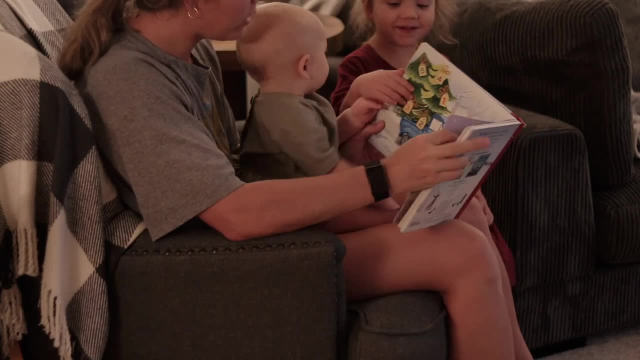 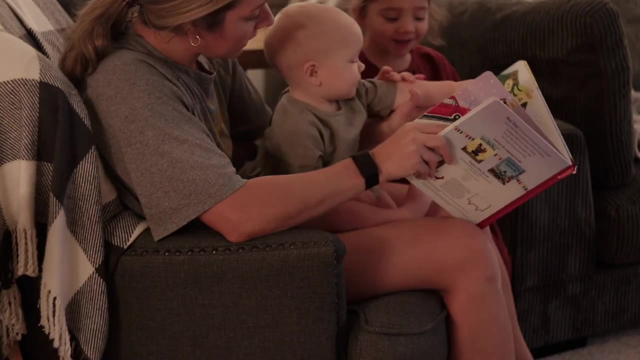 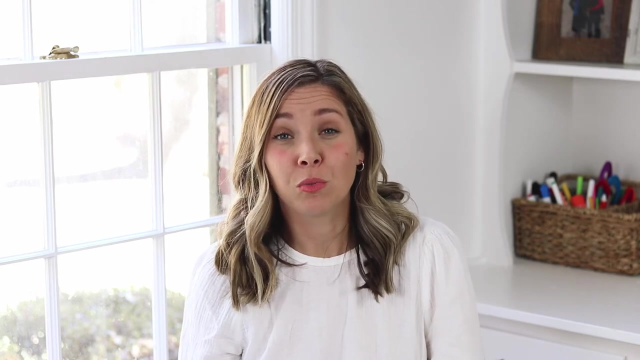 to show for at the end of the day. if you've read to your baby, if you've prayed over your baby, snuggled your baby, just looked at your baby, slept with your baby, If you fed your baby and changed no boxes to check, even if your husband can't see your hard work, The Lord knows what you do when. 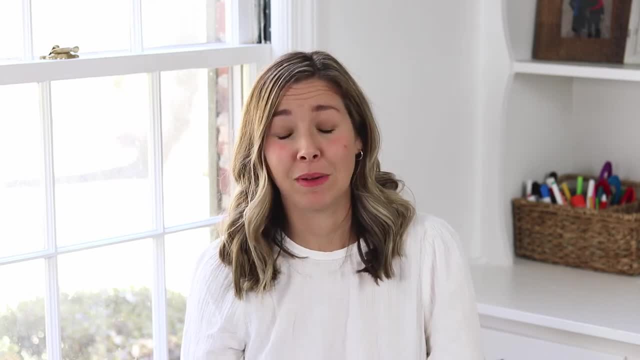 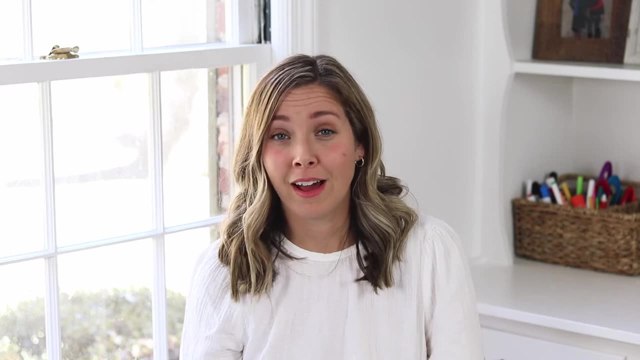 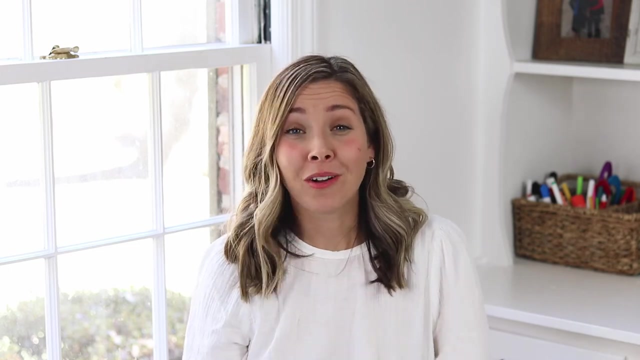 you're at home by yourself with your baby and it matters to him. It really matters to him. There are beautiful things done in the unseen that maybe the world doesn't hold up on high and maybe there's not a beautiful Instagram photo for, but it matters and it's beautiful to the Lord, and so I want to. 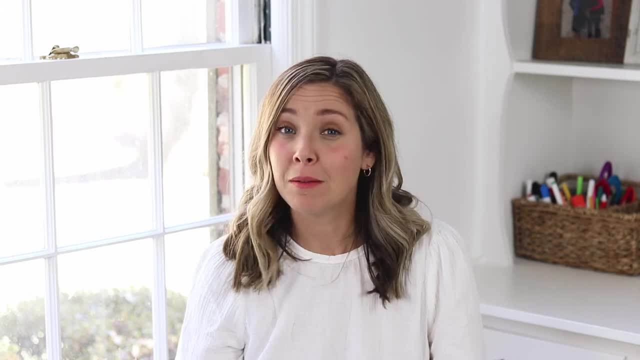 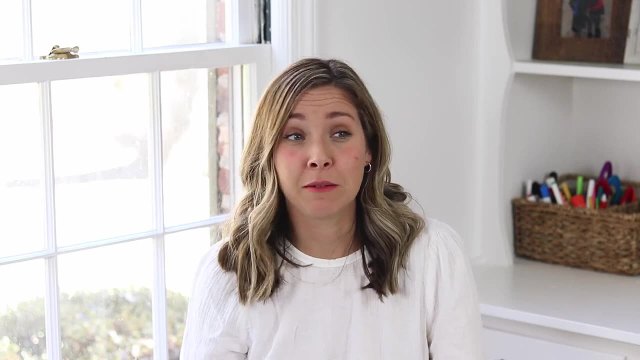 say: you are doing good work and don't give up. Keep planting those good seeds and you will reap a harvest. You really are going to reap a harvest. You're going to get better at this over time. This is a new job for you and you've never done it before. You're going to get better. You're going. 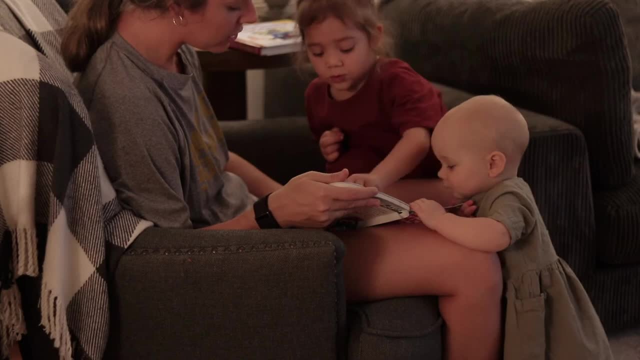 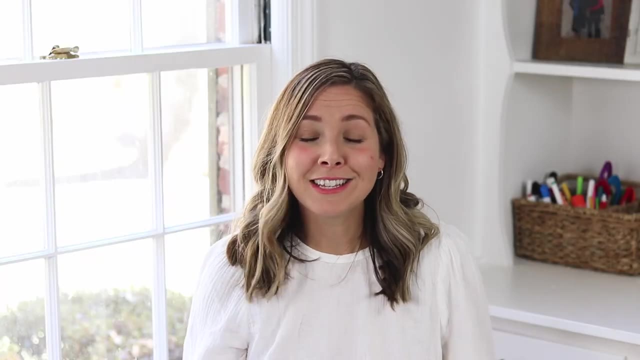 to get better if you just keep going. So don't give up, Just keep going. I want to encourage you. You've got this If you've never taken care of a baby before. it's a big new job and nobody's good at their job. 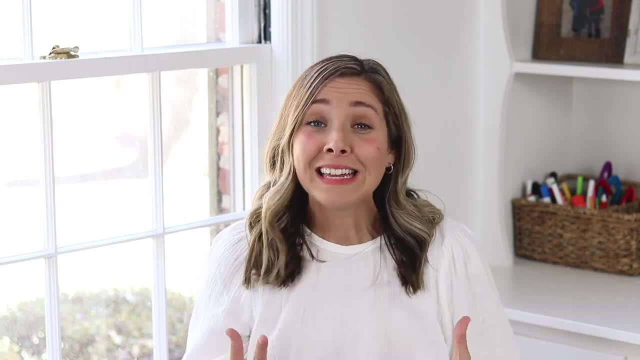 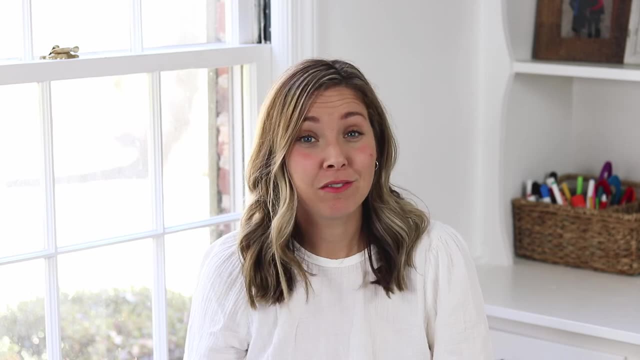 So just keep going. You've got this, So if any of this resonated with you, I hope you'll consider hitting subscribe. I would love to have you here at Girl Teach Me on YouTube, but I also love to have you at girlteachmecom, and thanks for watching this video. I'll see you again in the next one. Bye.